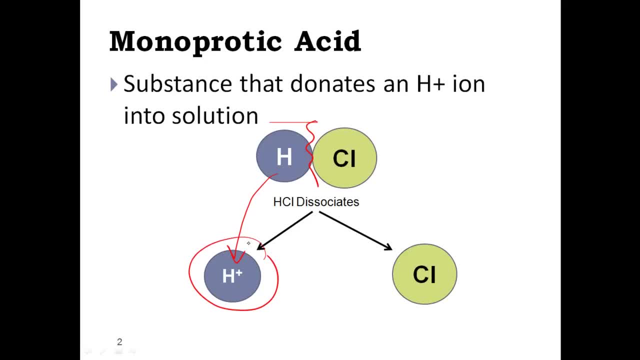 an ion, an H plus ion. Acids are substances that produce H plus ions into solution. So when we look at a pH, the strength of an acid is going to be determined by the quantity of H plus ions in solution, And for substances that donate just one H plus when they dissociate, they're called monoprotic. 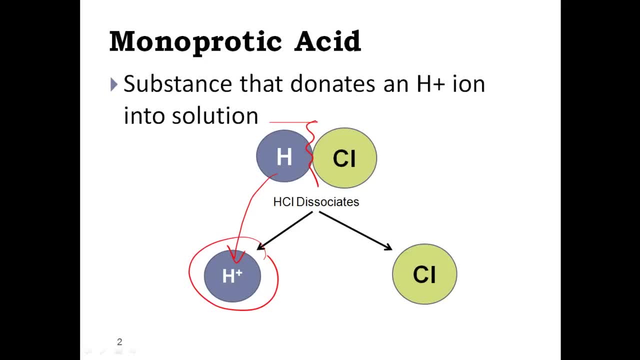 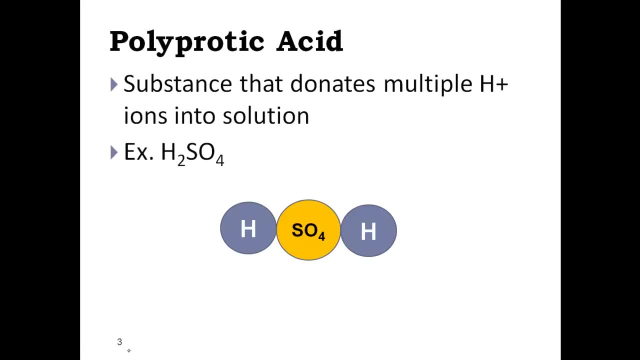 Now, for the sake of today's lesson, we're going to assume dissociation happens completely and that we're going to assume that all the acids we're discussing are strong acids. Also consider: you can have polyprotic acids. A polyprotic acid is an acid that donates multiple H pluses The one I. 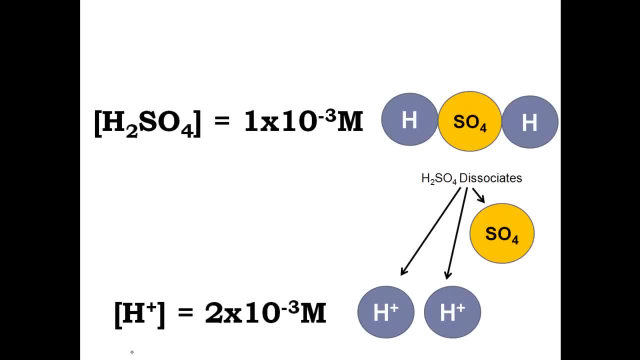 give you here as an example is H2SO4.. It's going to donate two H plus ions into solution, So that's two H plus ions when it dissociates. Just a little FYI, though, check this out over here. This is the. 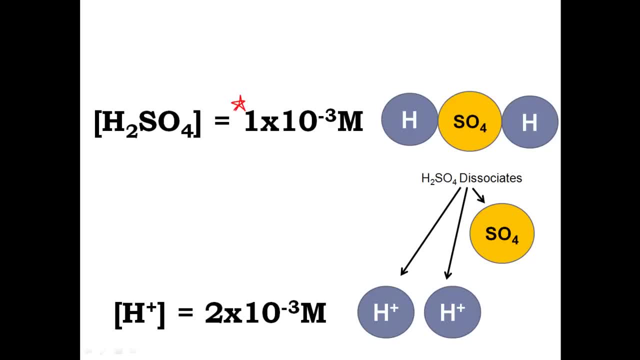 molarity of H2SO4. Let's just call it 1 times 10 to the negative 3 molar, which is 0.001 moles per liter of H2SO4.. Alright, that's one and the same scientific notation and just a regular expression. 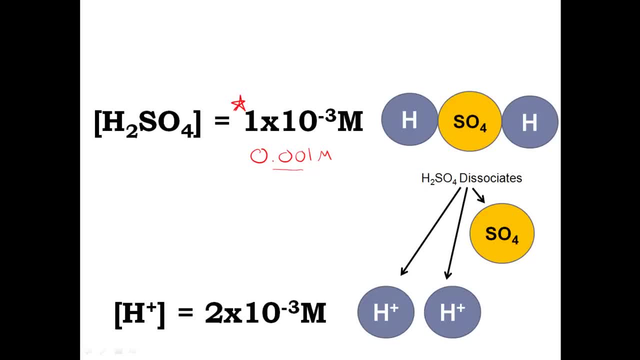 of it When it dissociates, though- this is really important for you- the H plus concentration of the H plus. So it's going to be one H plus ions when it dissociates. So that's two H plus ions when it dissociates. Just a little FYI, though. check this out over here. This is the molarity of H2SO4.. Let's just call it one times 10 to the negative 3 molar, which is 0.001 moles per liter of H2SO4. 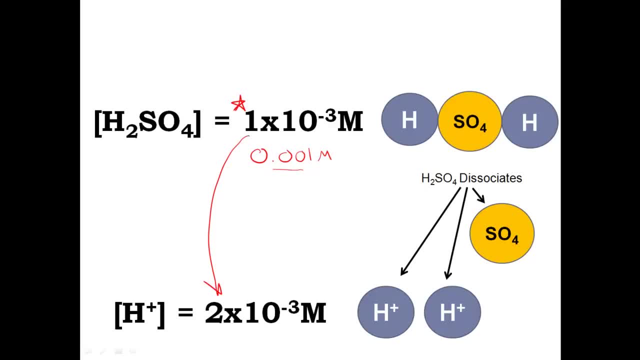 doubles. The ion concentration is double in this example because you have two H's that are dissociating, All right, so that's huge. One H2SO4 will produce two ions of H plus, therefore doubling the ion concentration. Remember, we're talking today about pH, and pH is all about the 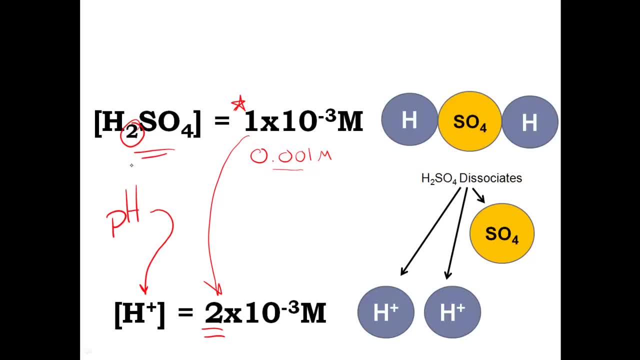 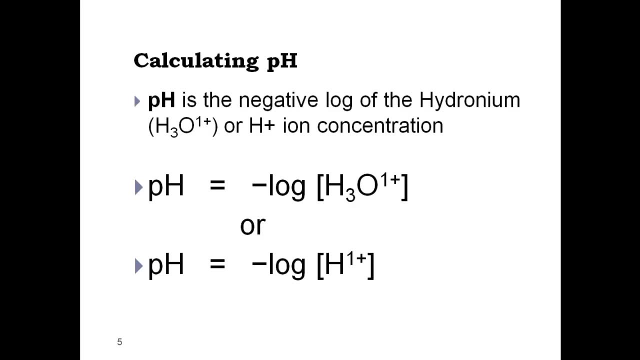 concentration of the ion. It's not necessarily as much the concentration of the H2SO4.. You want to be reminded that it's of the H plus ion. All right dudes. the formula for pH is the negative log of the H plus ion. Also, we could express it as the hydronium ion, which is the H3O positive. 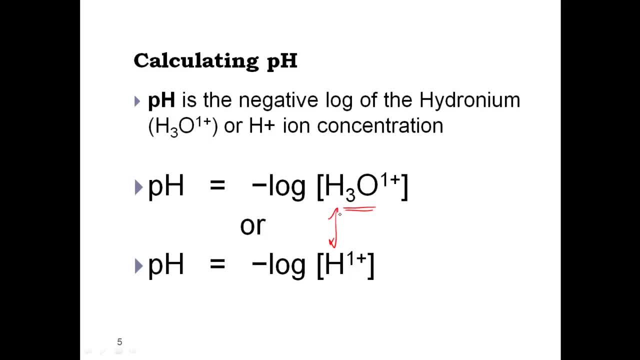 ion. So we're going to use these interchangeably. In a sense they mean the same thing. I don't want to go into a lesson on the H3O plus ion, but basically we're talking about the same exact thing here. So we're looking at the negative log of that hydronium ion concentration. 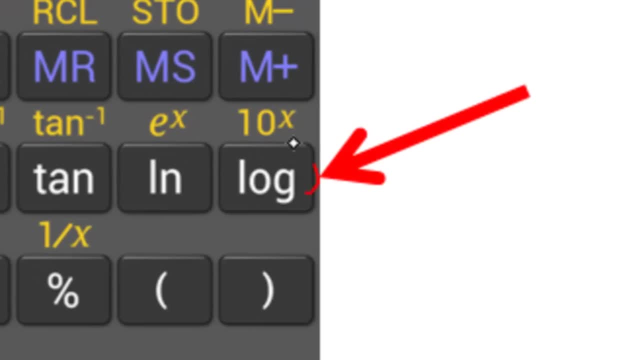 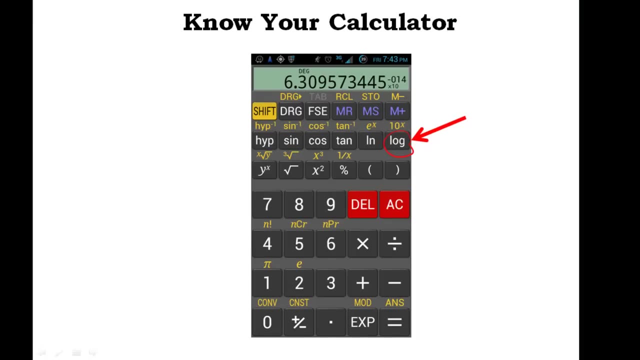 Know your pH Calculator. calculator Calculator is huge on how you use it today. This is the button. Experiment with that right now. This is not a lesson on how to use your calculator, but you need to know how to use that button. okay, You're also going to need to know how to use this button right down. 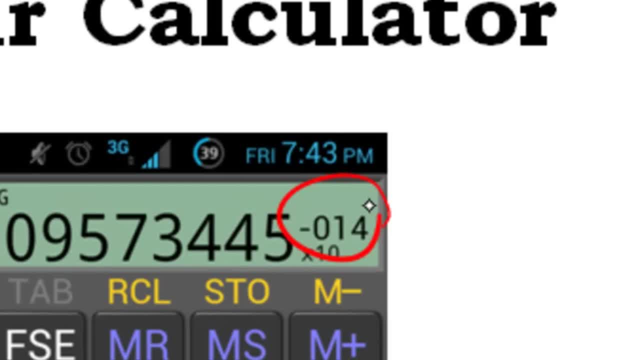 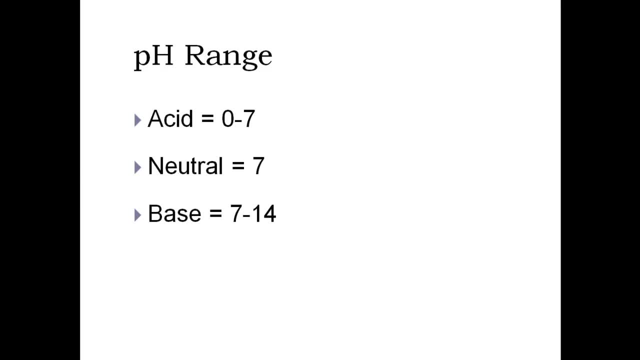 here the EXP button, because that's how you're going to get to that number right there. You need to use the EXP button. All right, dudes, here we go. Let's rock. The acids generally range in pH from zero to seven. A neutral solution will have a pH around seven-ish and a base solution from. 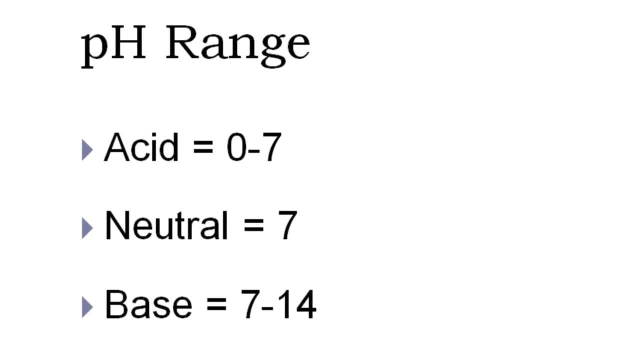 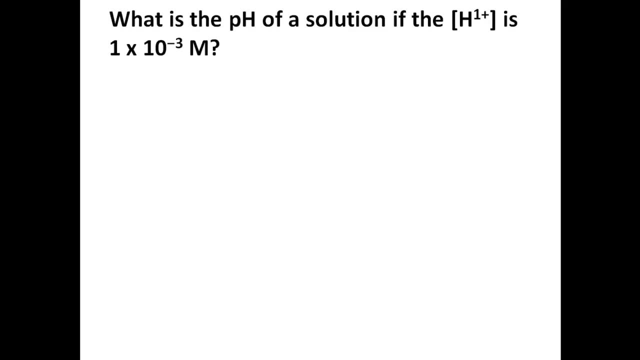 seven-ish up to five-ish, So you're going to need to know how to use that button right now. So these are the range of what's considered an acid, a base or a neutral solution. Let's rock and roll here. Here's the first question coming at you. We're going to use our formula. 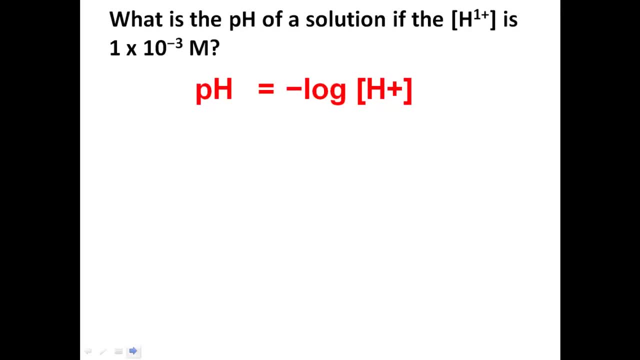 so let's plug it out there. The pH is the negative log of the H plus concentration. Let's go to the problem now. What is the pH? So we're looking for the pH of a solution if the H plus ion concentration, that is, after dissociation, is one times ten to the negative. 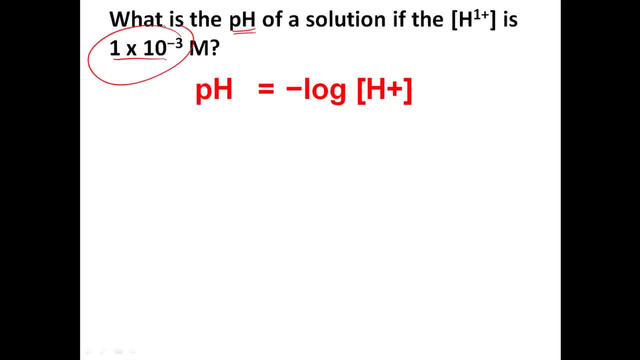 three. Here is the deal, dudes: You're going to have to plug in that number into here, All right, So you're going to be using your calculators now to plug the concentration of the H plus ion into here. These brackets that you see here, dudes, these guys, these things mean concentration. 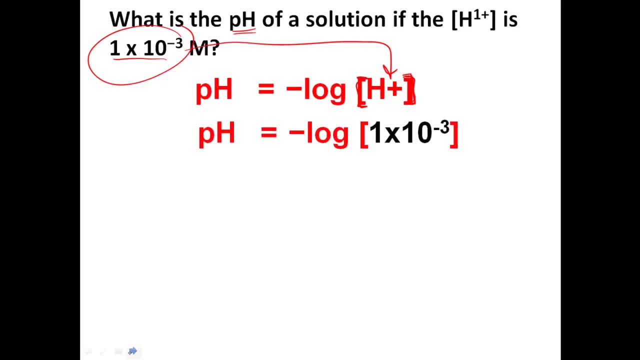 specifically molarity. because that's what we're doing in this problem. We're going to plug the number in and what you're gonna find- we take the negative log of that number- is that the pH is three. But let's just say if you ended up with a concentrate or the pH of negative three, just 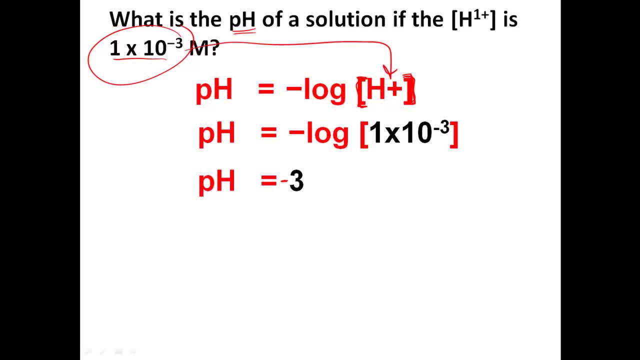 know that you need to make that positive. Not all calculators will allow you to use the negative log. That's okay. Just at the end go back and correct it because there is no negative pH. One little fine little note here. it's really cool. a little fun fact you maybe want to. 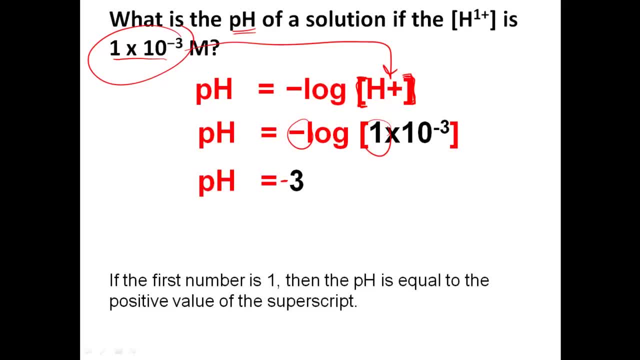 call it If the number is one, if that number is just one and not one point, something I want you to know this: The pH is always equal to the exponent value, but positive. So the pH is three. that means it was one times ten to the negative third moles per. 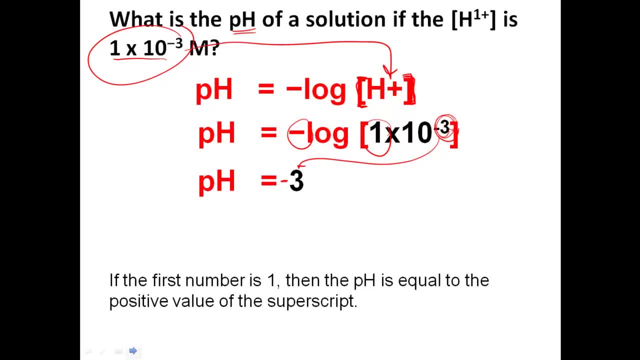 liter of concentration of the H plus ion. Let's try the next one Now, if you're really starting to groove. the thing I'm going to recommend is you press and pause. That's right. You press, pause right now. You try to solve the problem. 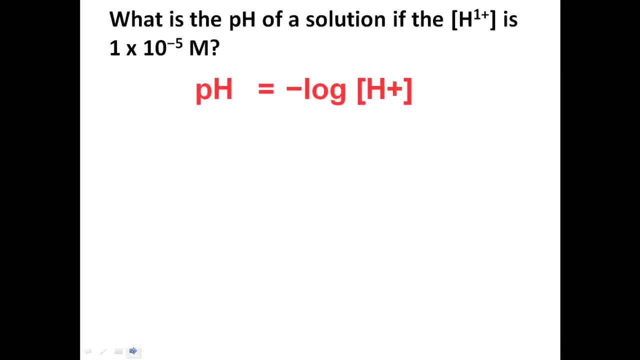 You know I'm coming back with the answer because here it goes. right now We're looking at this problem. We know it's the negative log of the H plus ion. Remember I said a second ago: Whenever it's a one little hint, you kind of know what the pH is going to be. 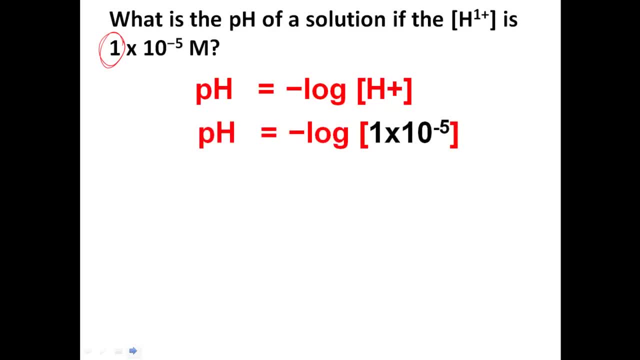 So take a guess what the pH is going to be. I plug my concentration in there and voila, I got myself a pH of five. That's right, dudes, Whenever my first number here is. one little fun fact is that my exponent will equal a. 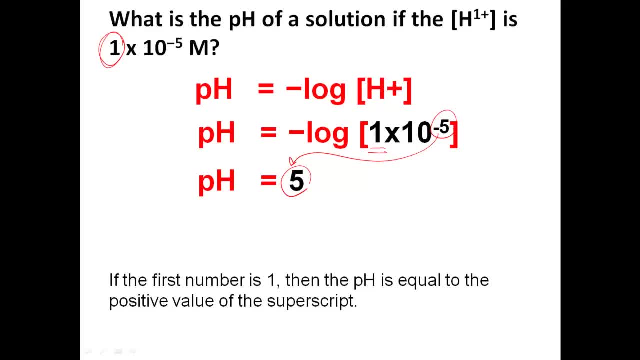 positive value in pH. That should be a little thing you need to tuck into your brain somewhere. Your pH down here is always, always, always going to be in the ballpark of that value, Always will be in the ballpark of that value. 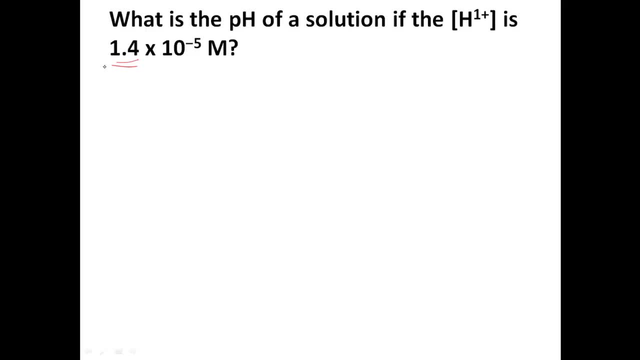 If I look at this problem here now, I'm changing it, I'm giving you 1.4, but I'm guaranteeing you something: For every single pH problem, your pH is going to be in that range of the negative five. 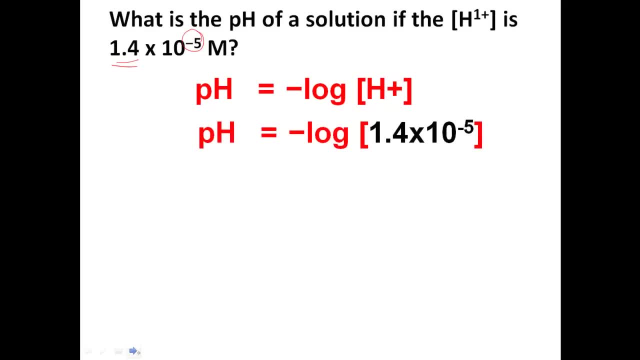 Let's prove it. dudes, Set it up, Do your substitution, Find the log of that, Change it to a positive. If it's negative, you're going to find your pH is in the ballpark of that negative exponent. right there It's 4.85.. 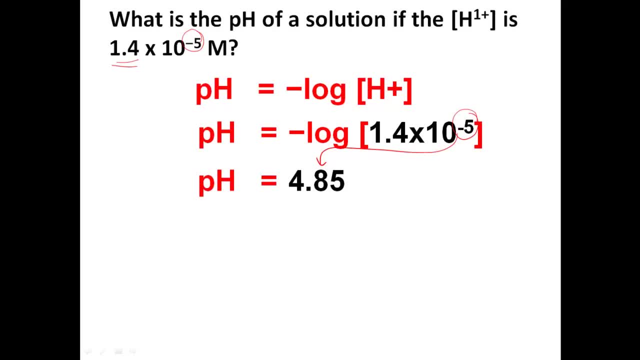 All right, dudes. What I'm going to ask you to do is that, if you're getting this, you want to go on to some of the slides coming up. You definitely want to hit on some of the slides coming up, because I do throw some difficult. 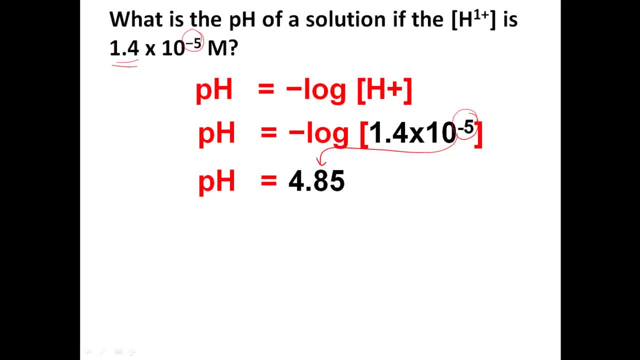 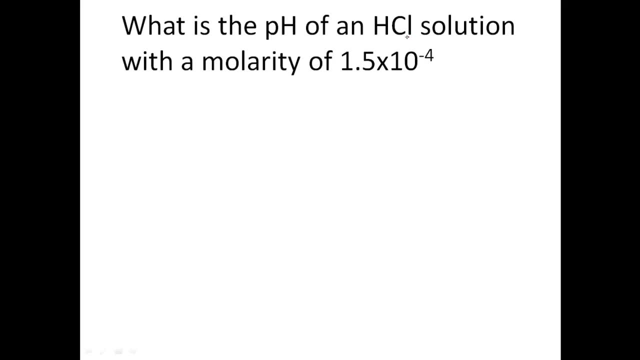 things at you. I want you to be skilled on All right dudes. so now I took away the H plus ion concentration and I'm just giving you here now a legit solution. This is a hydrochloric acid solution and the molarity of the solution is 1.5 times 10 to. 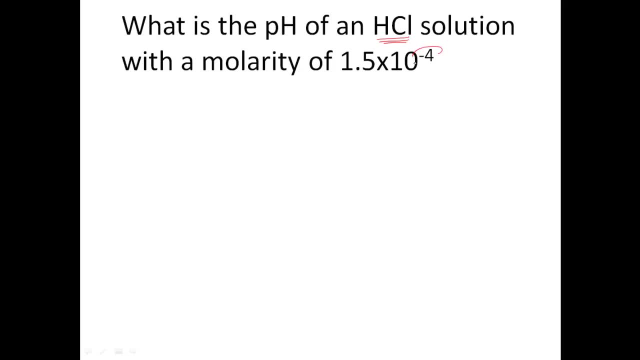 negative. fourth, Right off the bat, You're sending yourself the ions concentration because it is monoprotic. I have one H that will dissociate Key here. Now that I've given you actual compounds, you need to find out whether or not that acid 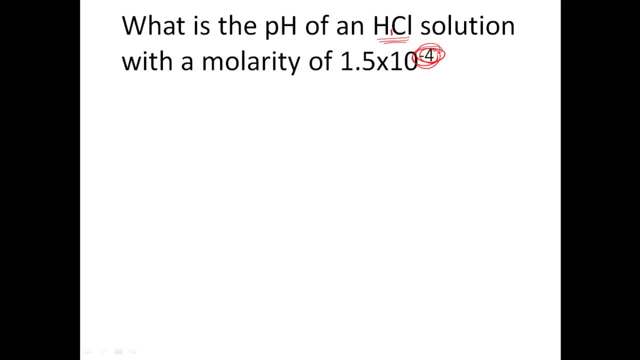 is monoprotic or polyprotic. Well, the pH, regardless, should be in that between the three to four range Should be in the ballpark of four. Let's plug and chug dudes. When you plug the number in, chug the answer out, you find it is in the ballpark of that. 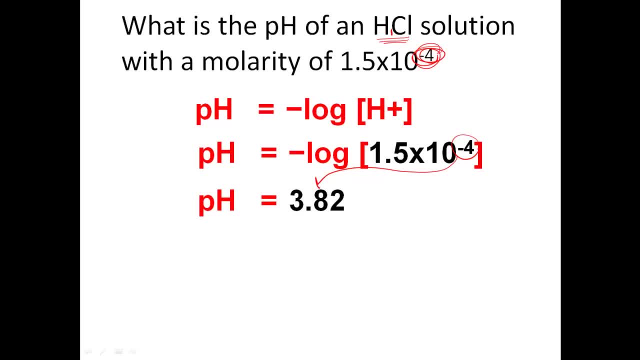 negative exponent 3.82.. Now, that was easy. All right, That was cool because it was a monoprotic acid. a monoprotic meaning one hydrogen is given off when it dissociates. All right, dudes, check it out. 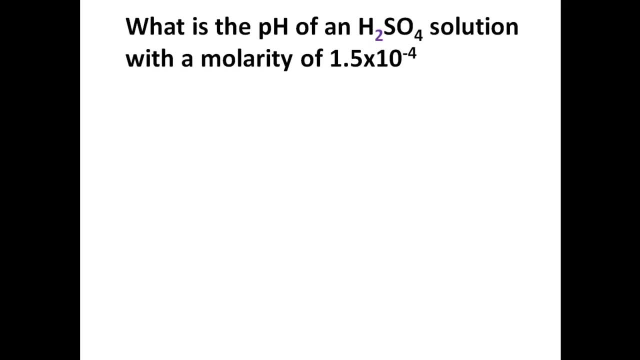 See if you can see the curveball that I'm throwing at you in this problem. If so, press pause. Just press pause and do it on your own, because here I come. All right, dudes, you're hitting a home run right now. 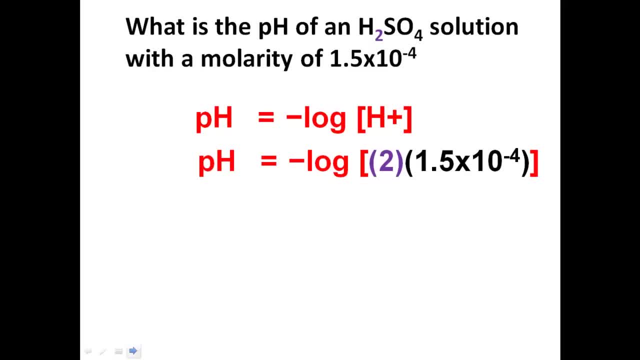 You are knocking the ball out of the baseball stadium. if you said and recognized that this was a polyprotic acid And I gave you the solution of the H2SO4. I did not give you the concentration of the ion. This is all about the hydrogen ion and solution. 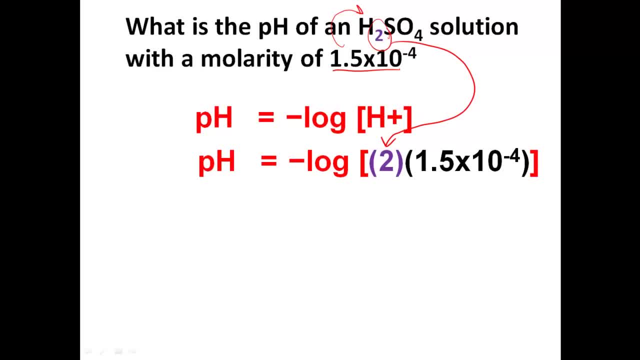 You double it because when H2SO dissociates we're going to produce two hydrogen ions. So two times 1.5 times 10 to the negative fourth is going to give me a three times 10 to the negative fourth. That is the number. 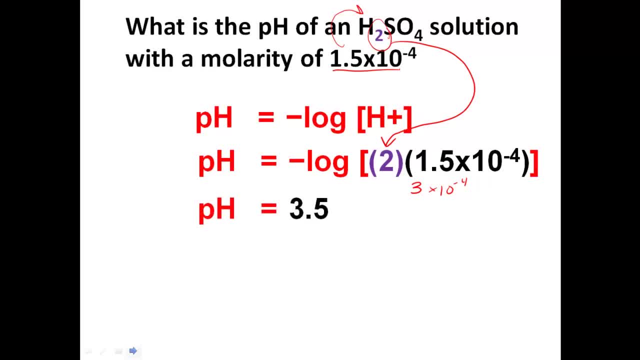 I'm finding the negative log of, and when I do so, dudes, you find out. yeah, you're back in that ballpark again. You're back in the ballpark of negative four. You've got a pH of 3.5.. 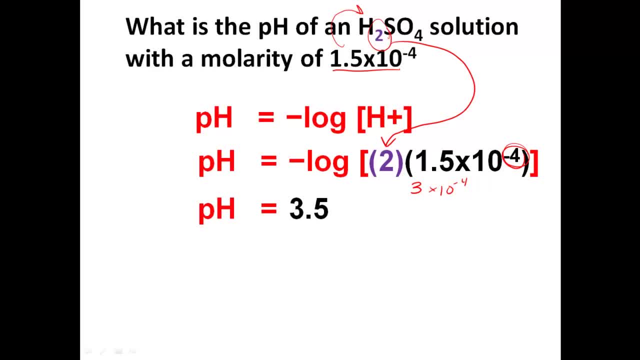 Now, if you had a pH of 2.5, I'd be a little concerned, because we still want to be within the range of that number right there. Good job, dudes. if you snagged that one, All right, next one: 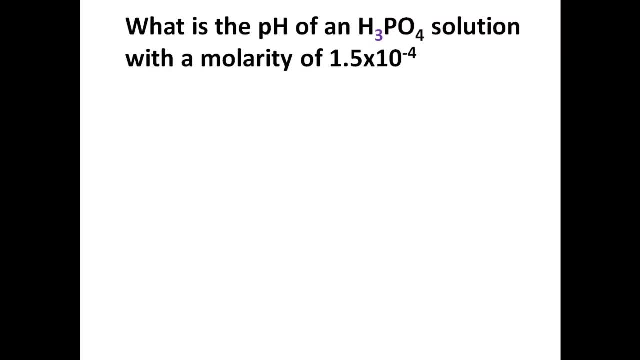 I'm throwing another curveball at you. Your job is to figure it out. Press pause, Solve the problem on your own. All right, dudes. here's what we've got going on. I start out with the formula. I make my substitution, but I want you to recognize, in this polyprotic acid I have 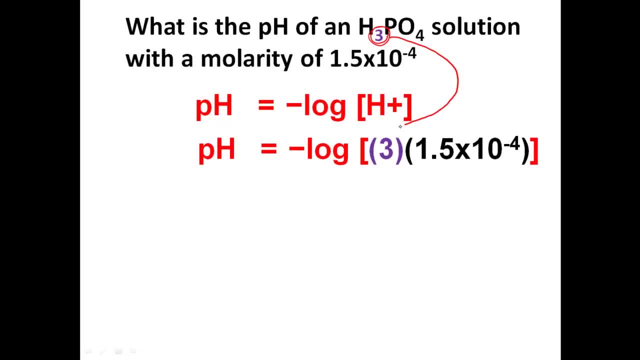 a three right there. so therefore, I'm going to multiply the concentration of the acid, because I have three times that concentration of the ions floating around in solution. It's those active ions that's going to cause my solution to be more acidic. That's what we're seeing here, because when we plug the numbers in, it was less than last.